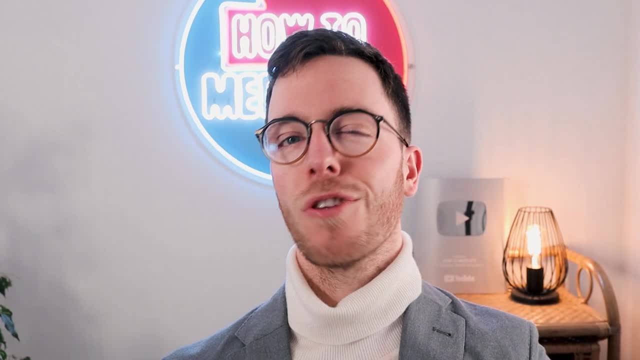 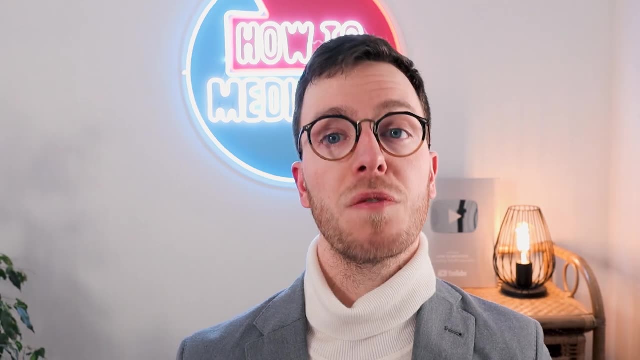 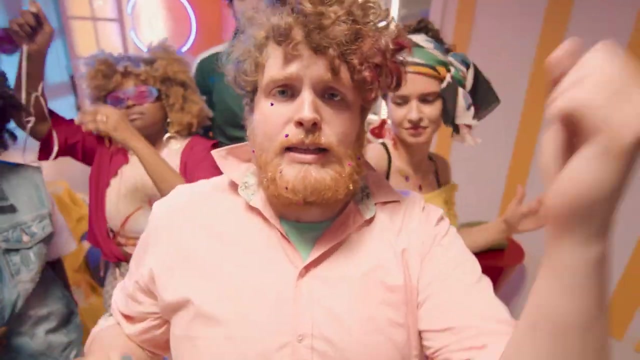 Intro. So let's start at the beginning, The origin story of nitrous oxide, which is a lot older than you might think. It was for the first time synthesized in 1772 by a guy named Joseph Priestley, And it took us, humanity, only 29 years to explore its recreational properties. 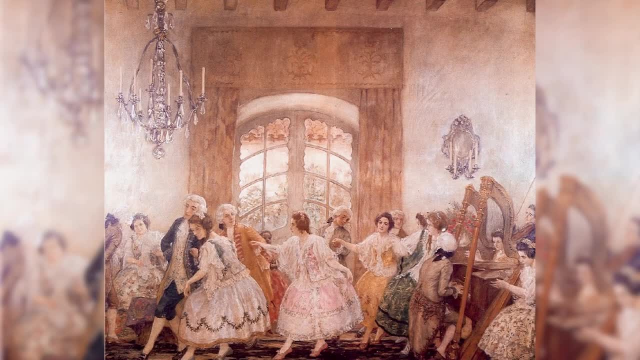 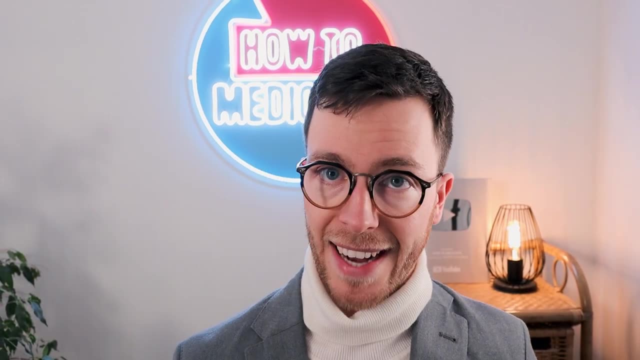 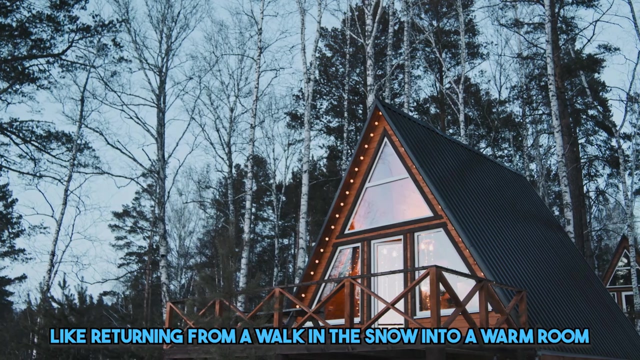 By 1799. it was the latest craze for the British upper class. You can picture them in lavish parties consuming the nitrous oxide in silken bags, And a poet from that era described its usage as like returning from a walk in the snow into a warm room. And to make matters even worse, 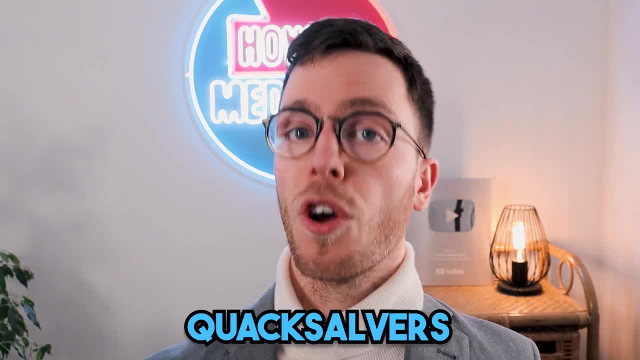 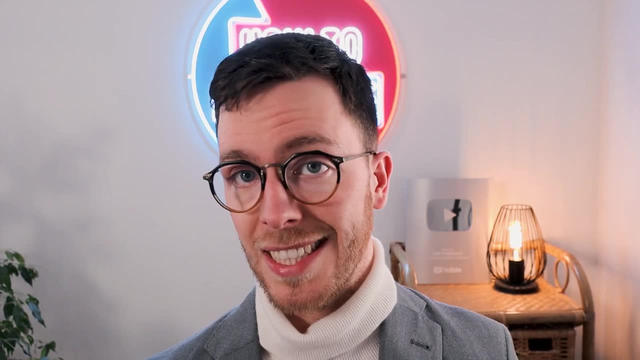 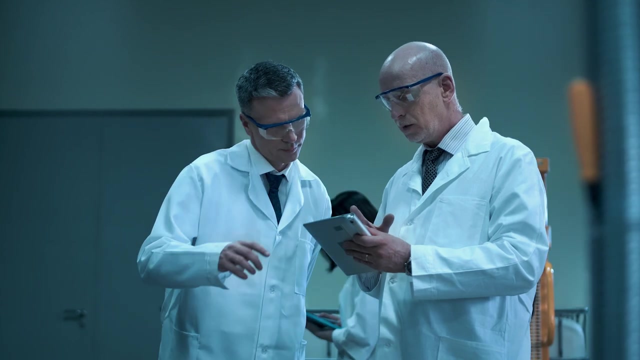 this gas also became popular among quacksalvers, which were fake doctors. They claimed all kinds of medical properties- It could cure blood, throat or lung diseases And unfortunately it were just death claims. In the years that followed, doctors and scientists, doctors and 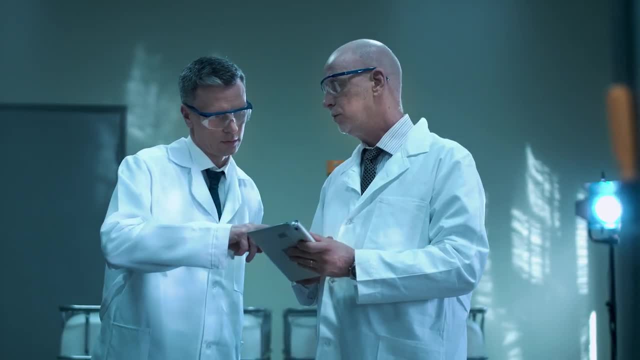 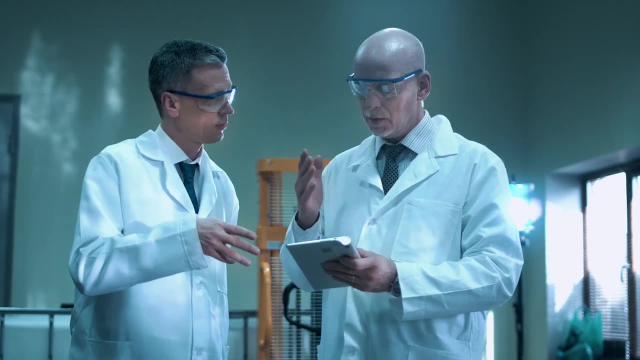 scientists started to develop scientific methods to examine the actual effectiveness of medicines, And the previously claimed medical properties of nitrous oxide seemed unbased. However, as you might know, in more recent times nitrous oxide got a place in the medical world. 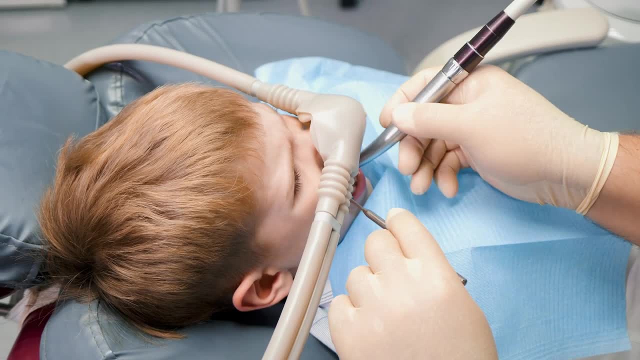 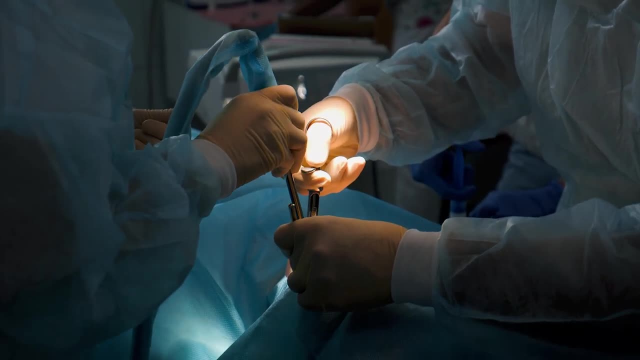 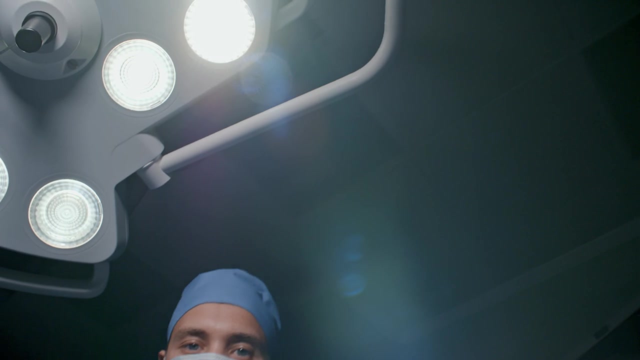 namely as an anaesthetic. It was first used by the dentist Horace Wells who demonstrated it could cause insensitivity to pain during a dental extraction in December 1844.. At first of dentists were full criticism and they were doubtful, Though with time more evidence was. 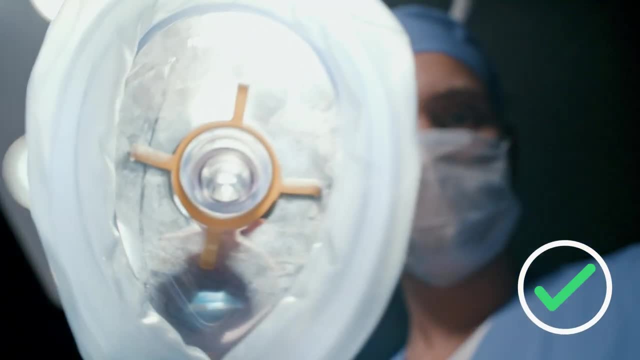 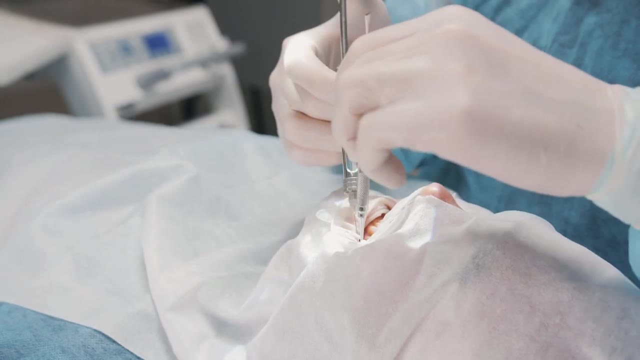 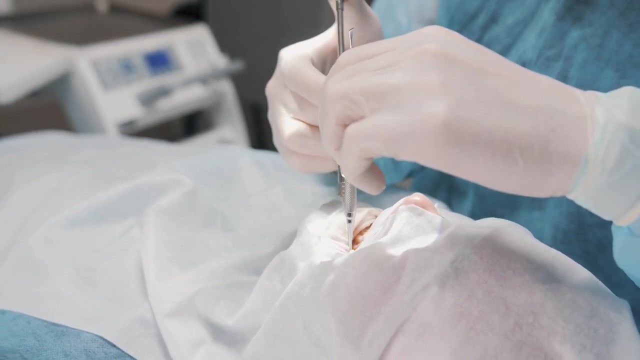 gathered and the method of usage was improved, And by 1863, it had come into general use. Today, nitrous oxide is used as an aesthetic and an anxiolytic, which is a drug that can be used to reduce anxiety during an inpatient and outpatient surgical procedure And beside its implementation. 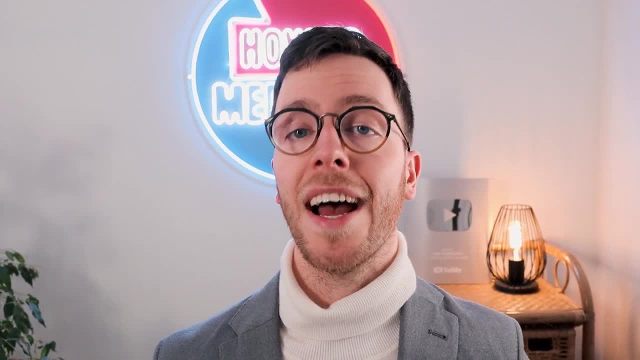 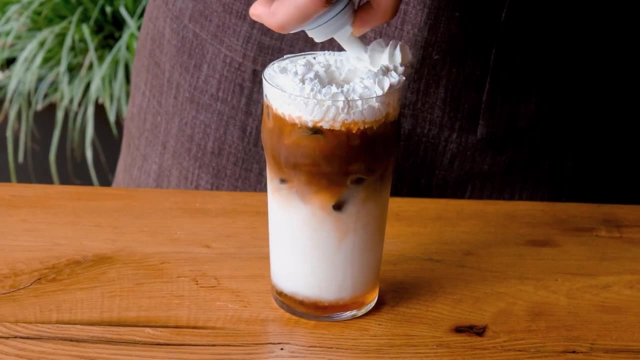 in the medical world. it was found that nitrous oxide was also very handy to make whipped cream. It could be used to prepare whipped cream and for that purpose it is sold in gas cylinders to restaurants. And of course these gas cylinders made its recreational use explode. 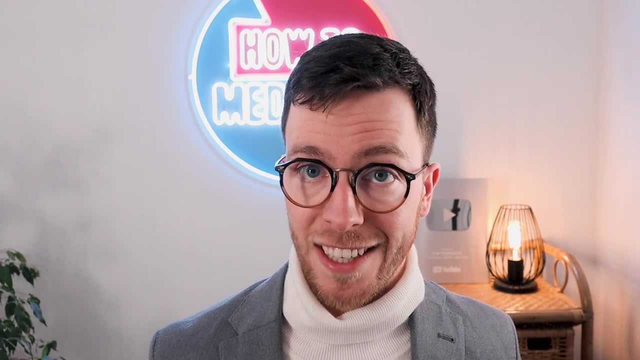 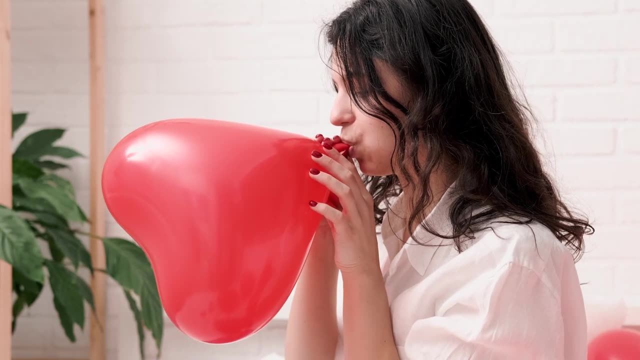 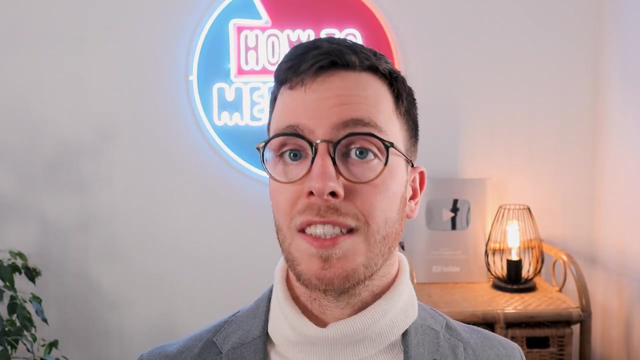 Again, as they are cheap, available and illegal in most countries. Thus a few which go clubbing or visit a rave once in a while have seen its popularity There. this drug is often sold in balloons filled with nitrous oxide. Altogether, this makes nitric oxide besides cannabis. 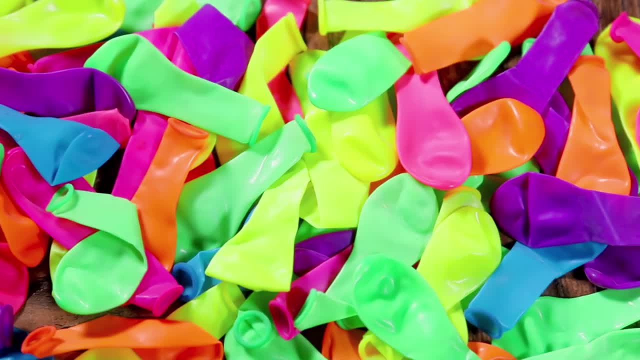 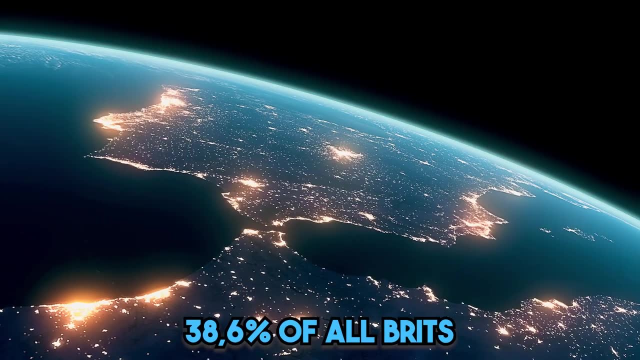 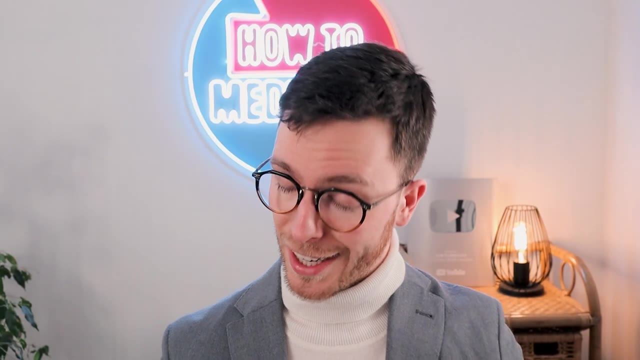 the most used recreational drug in the world. In 2014,, Global Drug Survey found that about 29.4% of all Americans and 38.6% of all Brits have used nitric oxide at least once in their life. This is a lot of people, But its numbers get even more extreme If you find someone who went. 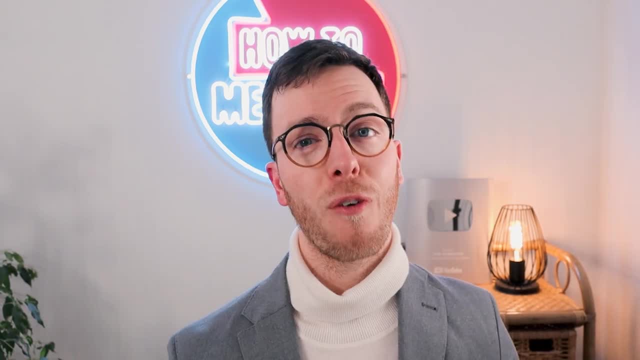 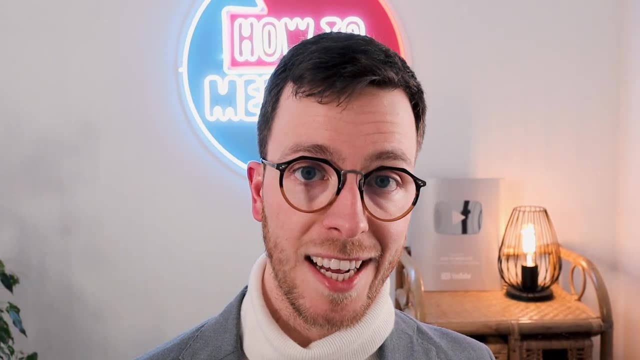 to a rave or a party this last month, there is a 40 to 80% chance that he or she has used nitrous oxide, Which brings us to the drug itself. Nitrous oxide is also known as NOS laughing gas, nitro. 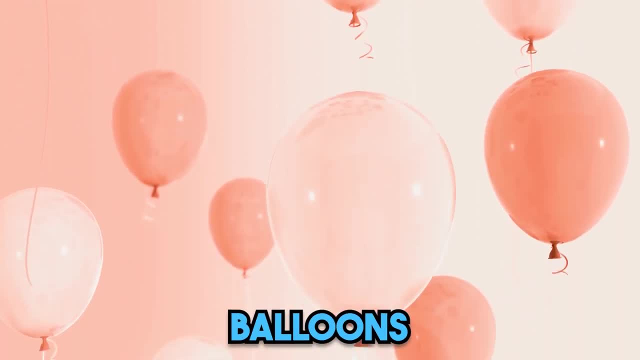 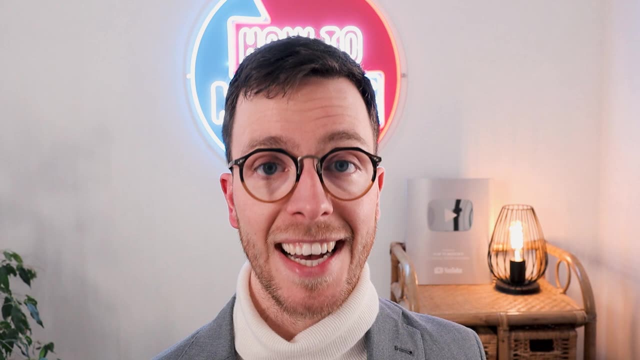 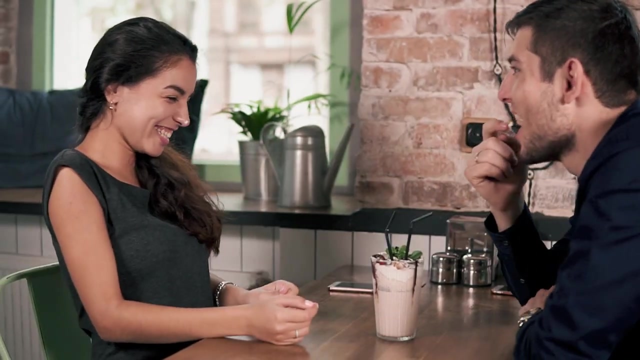 nangs, whippet, hippie, crack bus, bombs and balloons. As mentioned, it's a chemical compound with the structure N2O and at room temperature it's a gas. it's non-flammable and it has a slightly sweet smell and taste. For recreational use, the gas comes in a canister or cylinder. 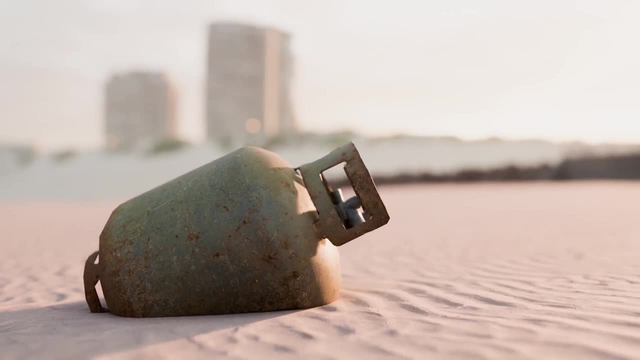 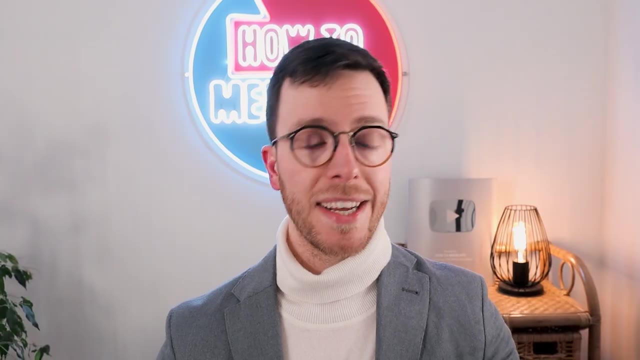 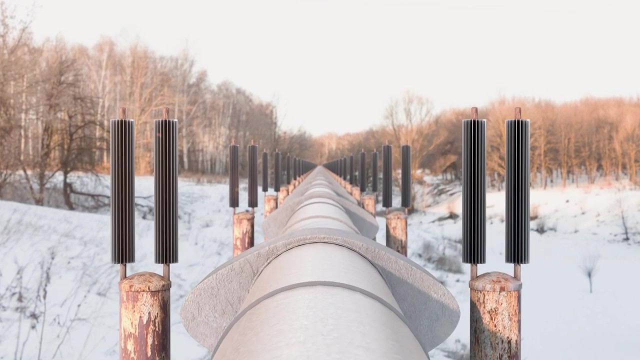 called a whippet. These contain about 8 grams of nitrous oxide, or the gas comes in a big tank. These are used to fill balloons or whipped cream dispensers. From there the gas is inhaled directly: from the dispenser or from the balloon. This is necessary because the gas can get very cold under. 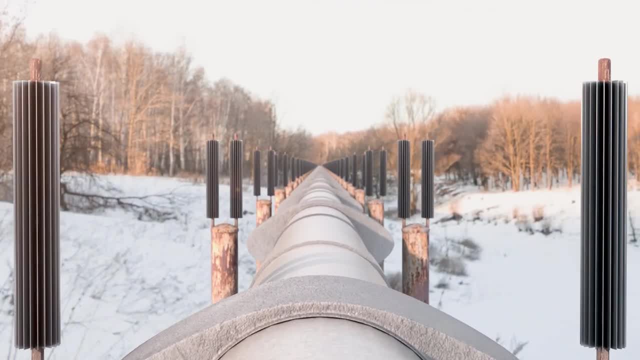 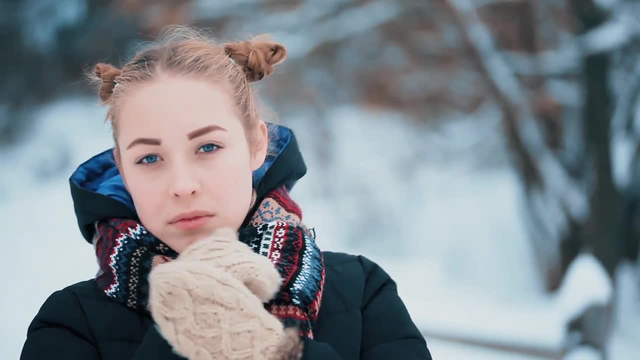 extreme pressure when it exits the canister or the tank. Inhaling it directly from the tank could be very dangerous because it could cause a severe frostbite of your throat, mouth and lungs. When you're inhaling the whippet, the gas comes in a canister or cylinder called a whippet. These are 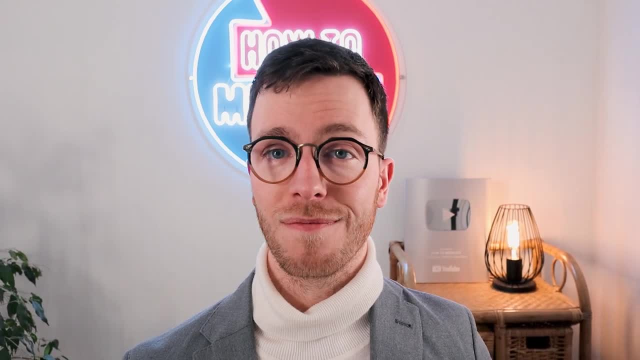 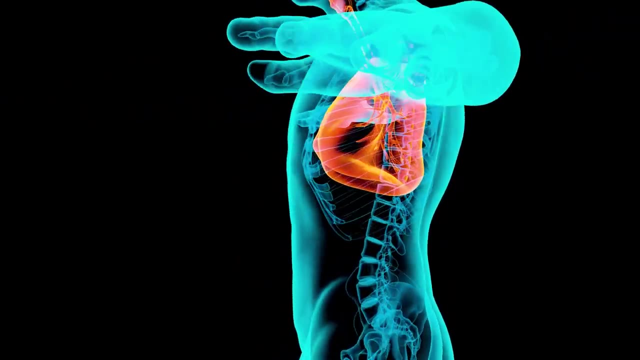 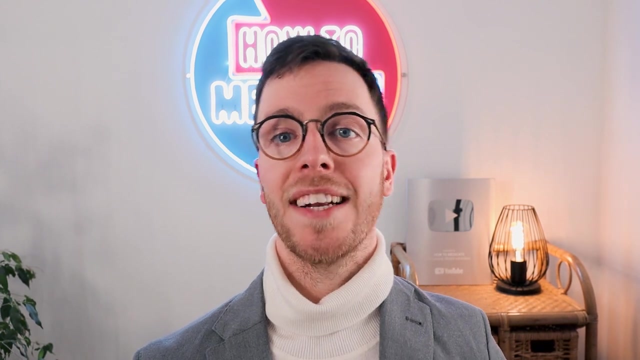 the gas from the balloon that enters through your mouth into your lungs. There it is absorbed by your alveoli, which normally exchange oxygen and carbon dioxide during the process of breathing in and breathing out, And your alveoli are able to do this almost instantly. That is why nitrous 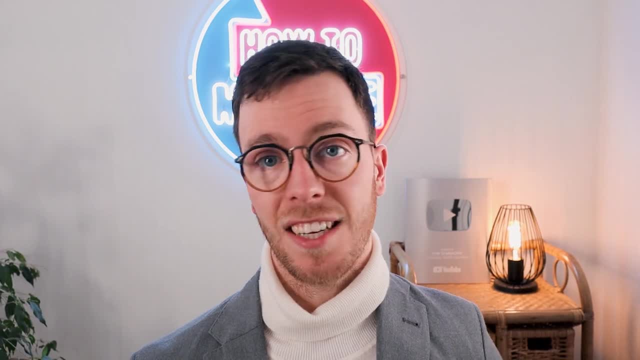 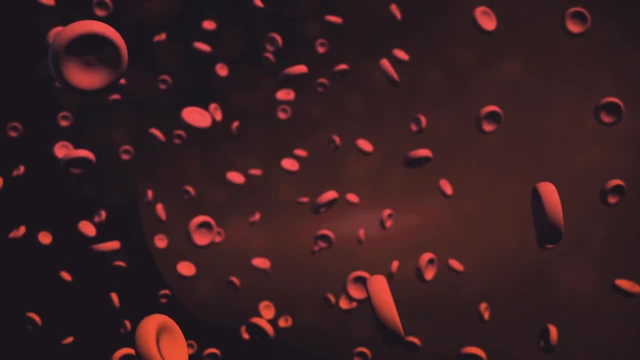 oxide works almost immediately as well, and its effects last for about one to two minutes. From your lungs, nitrous oxide enters your bloodstream, and there it binds to multiple receptors in your cell. This is why it's called a whippet or whippet, because it's a gas that 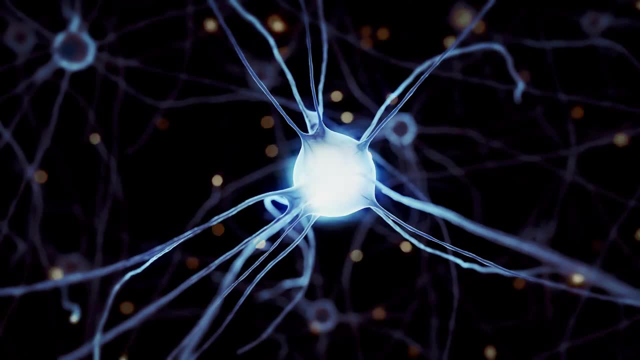 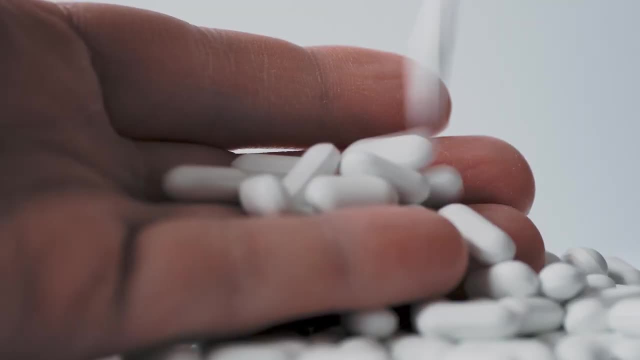 enters through your lungs into your central nervous system. Its anaesthetic effects come from binding to the NMDA receptor, which causes your body to release opioids. These cause a similar effect as the drugs morphin would cause. Nitrous oxide can also bind to the GABA receptor. 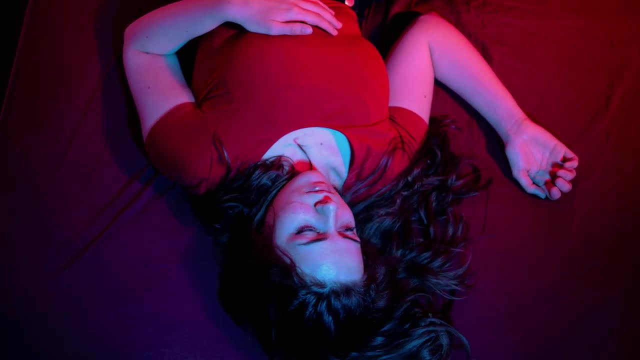 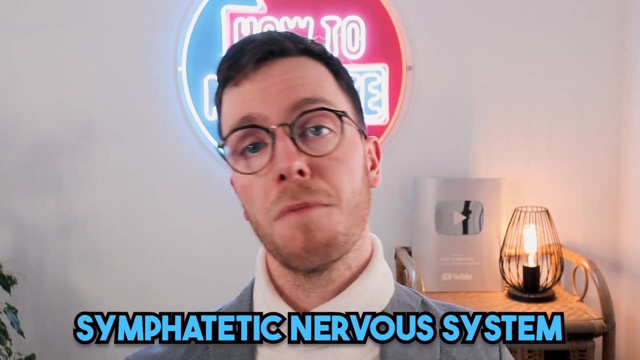 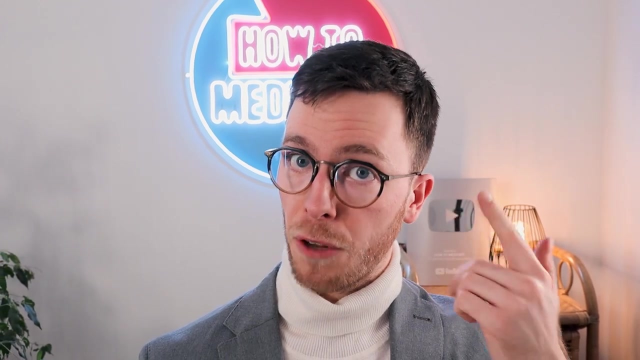 which has an inhibiting effect on most of the brain pathways, creating an anxiety-reducing and calming effect. Nitrous oxide also stimulates your sympathetic nerve system. This causes your blood pressure to rise, increases the output of your heart, increases your intracranial brain pressure. 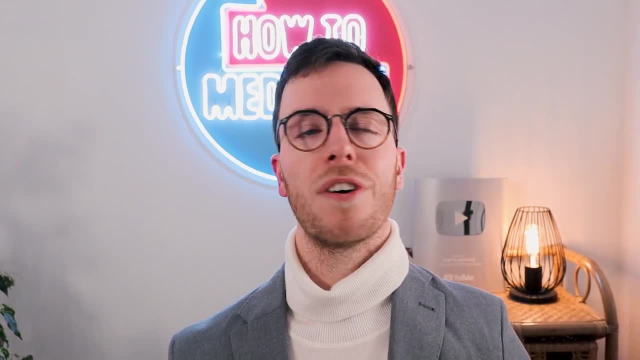 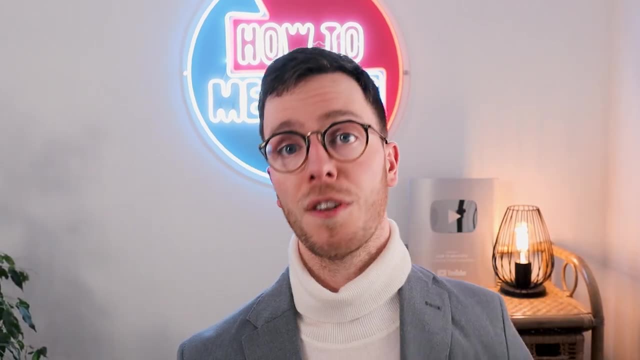 as well as the blood flow to your brain. Now you might wonder: what are the effects of nitrous oxide? Well, this depends. It depends on your tolerance for it, depends on the amount you take, depends on your size, your weight and if you combine it with any other drugs Here. 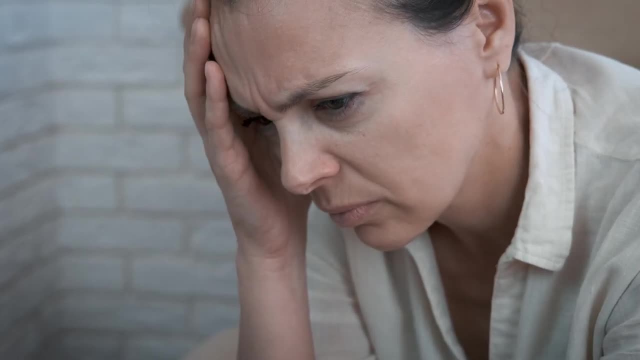 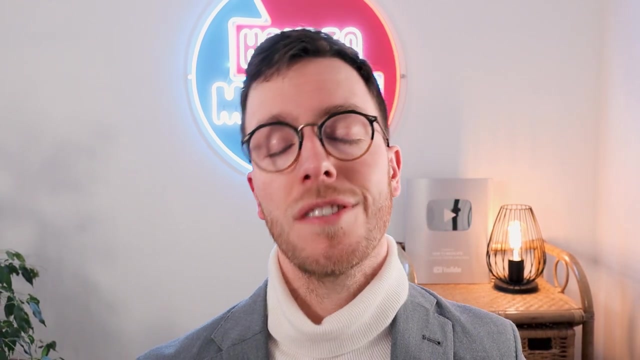 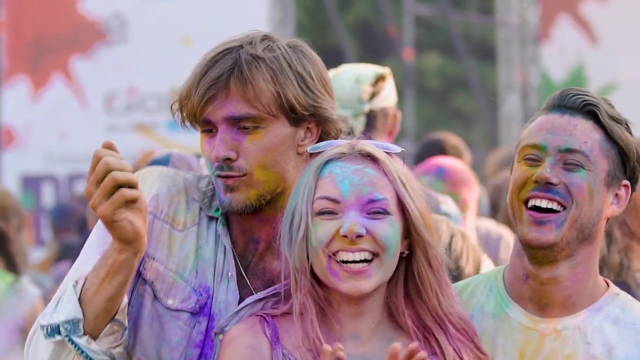 it is also important to mention that there is no completely safe level of nitrous oxide use. Using nitrous oxide carries risks, so take that and the previously mentioned factors into consideration. However, when using it, the potential positive short-term effects are feelings of euphoria. relaxation and calmness, giggles and laughter and hallucinations where you hear or see things which aren't really there. Unfortunately, it can also cause some negative effects, like a severe headache, dizziness, numbness of your body, sedation, uncoordinated movements, a blurred vision. 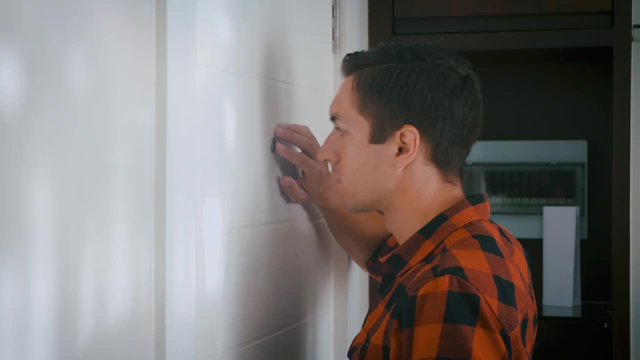 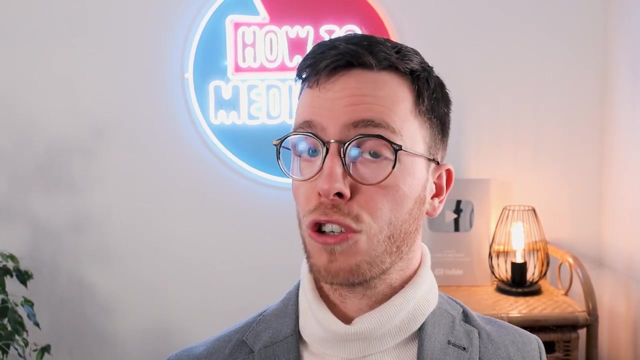 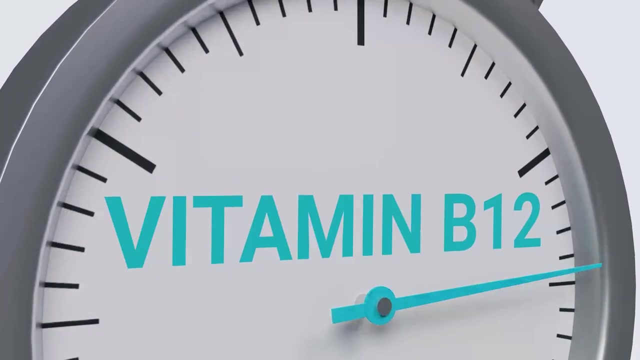 confusion, sweating, fatigue, feelings of paranoia, and it can prevent you from thinking straight. Besides these short-term effects of nitrous oxide, long-term use, especially when it's frequent or combined with other drugs, can cause serious health complaints. It can lead to a vitamin. 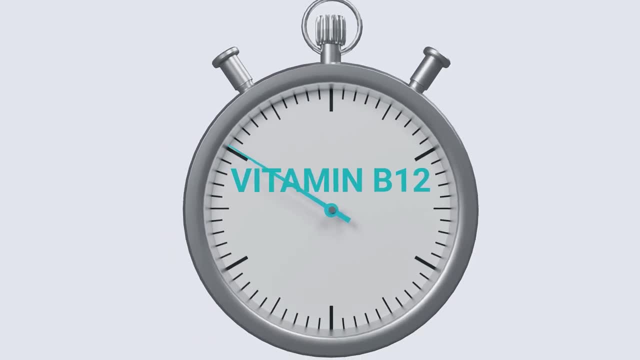 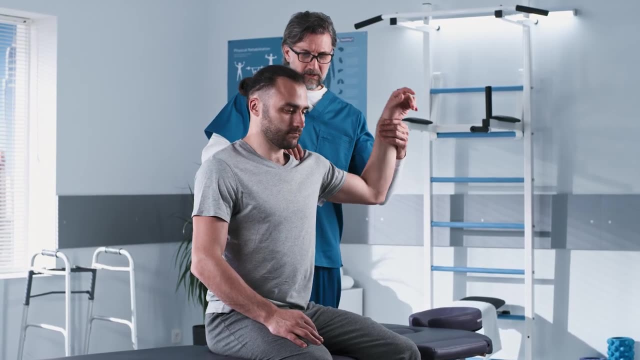 B12 deficiency, which could cause serious nerve damage. This can lead to persistent numbness and tingling in your body, mostly of your hand and your feet. This can be painful, cause problems with walking, driving and the usage of your hands. In extreme cases it can even lead to the development of a paralysis. Frequent usage can also lead to a specific type of anemia, where your body stops making a certain white blood cell. This can have an impact on your immune system. Other common health problems caused by the frequent and long-term use of nitrous oxide could be memory loss. 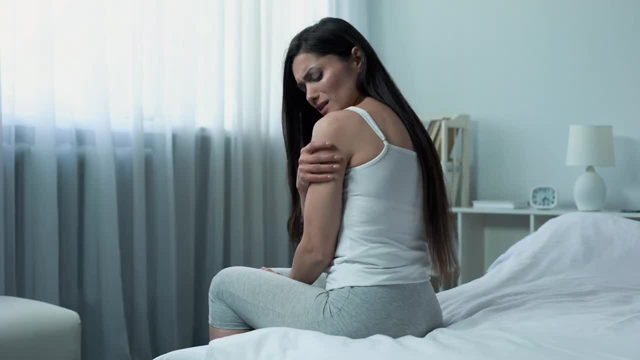 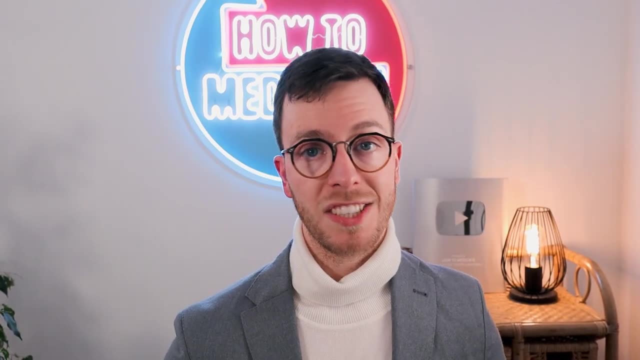 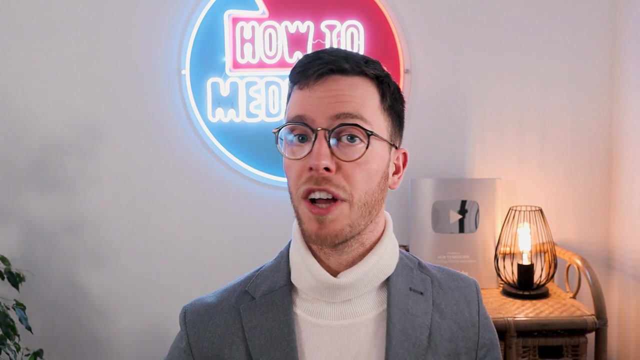 a ringing sound in your ears, incontinence spasms, potential birth defects if you use it when pregnant, depression and psychosis. Here it is important to mention that it is possible to overdose from using nitrous oxide. This is partly due to the fact that it is very hard to dose as you use it. 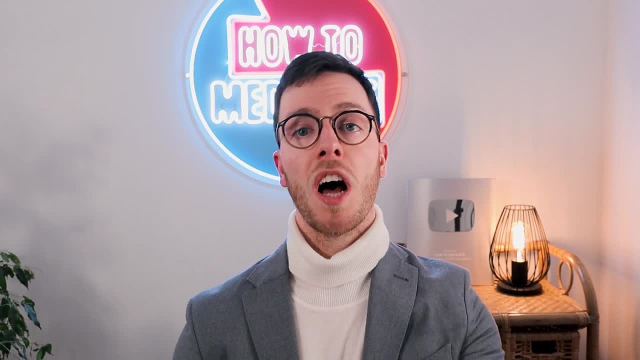 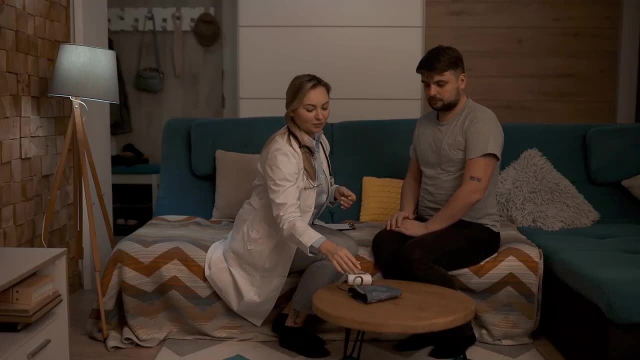 in balloons or canisters and you do not exactly know how much nitrous oxide you have consumed. This is part of the risk. When you have used too much, you are at risk for a lowered blood pressure, potentially causing you to lose consciousness, falling and having an accident. 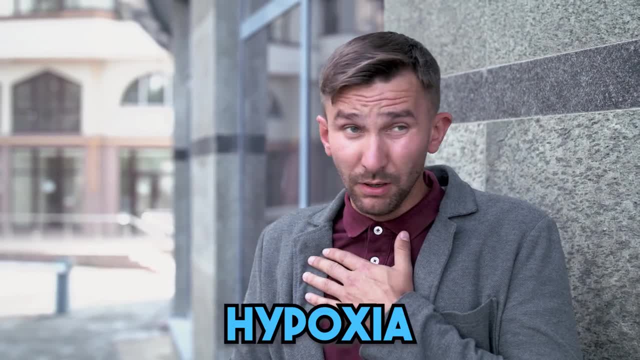 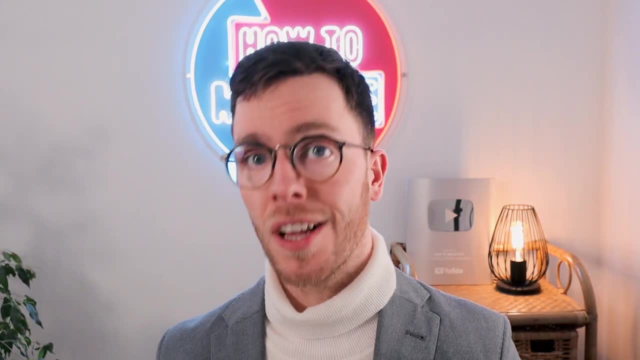 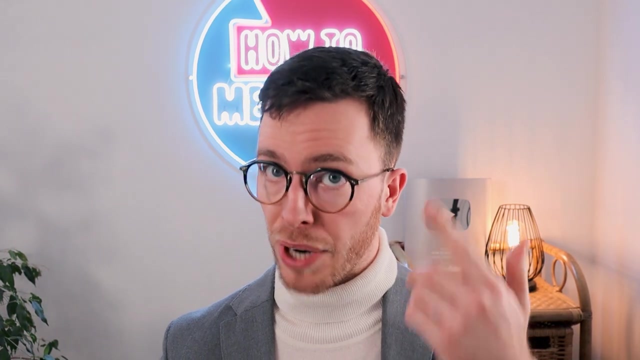 and or suffocating from the lack of oxygen due to hypoxia. This is a real risk, which could be further increased if you combine nitrous oxide with alcohol, as both activate the GABA receptor. As mentioned, activating GABA leads to an inhibition of most brain pathways. 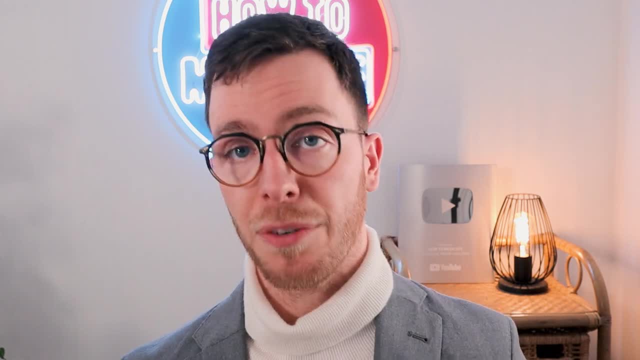 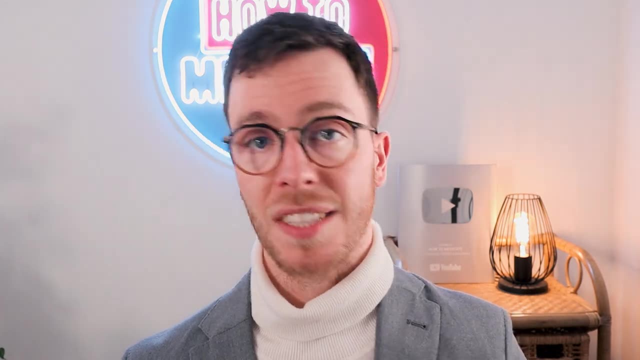 In extreme cases, this could lead to the inhibition of your breathing reflex. This can be a life-threatening medical emergency. So please, if you see any of these symptoms in anyone, please let me know in the comments below. Thank you for watching this video. If you liked it. 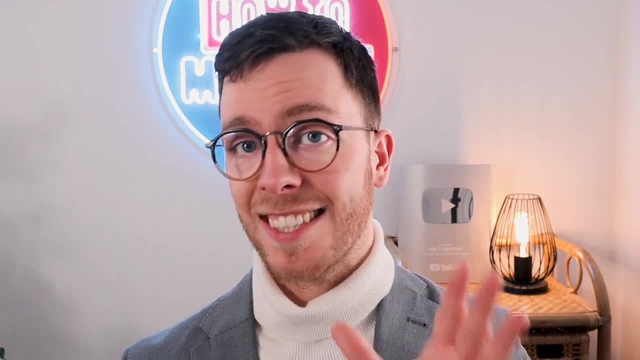 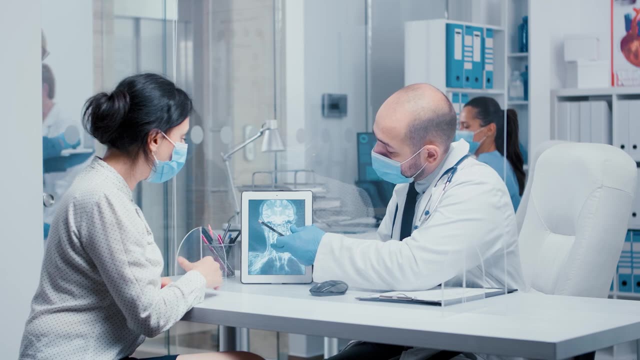 leave a like and don't forget to subscribe to my channel. See you in the next video. Bye, Call your doctor, call 911, call an ambulance, as this can save a life. Lastly, some practical tips which might help you to reduce your risk on serious health problems. 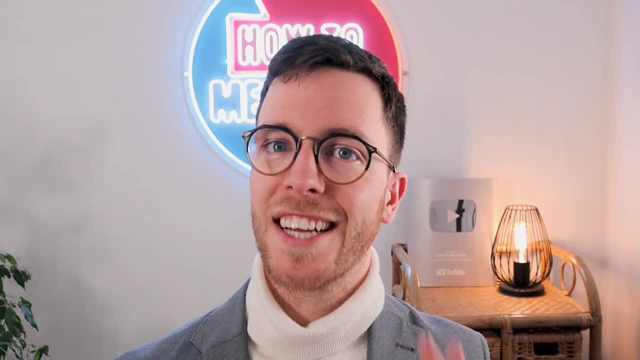 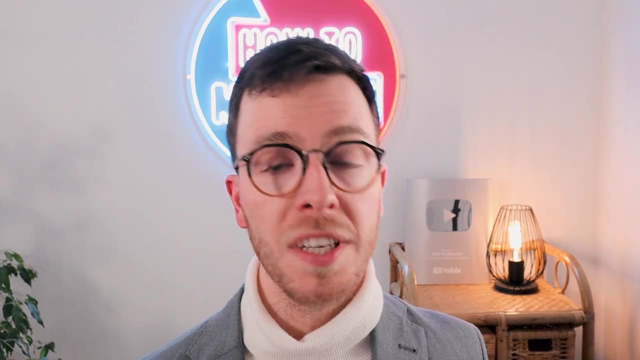 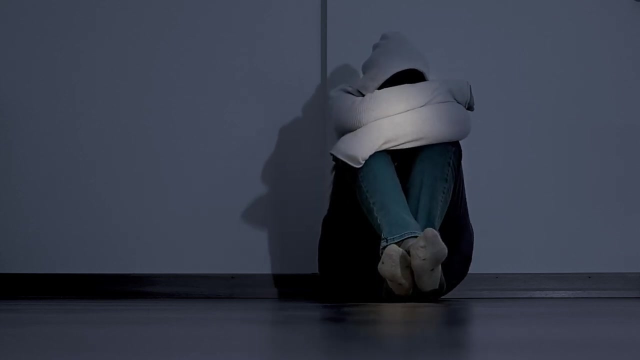 As with anything in life, moderation is key. The first tip is to always use nitrous oxide in a balloon. This will make it easier to know how much you have consumed and it will prevent these frostbite symptoms. Furthermore, it is also advised to not use it alone or in a dangerous or isolated area. 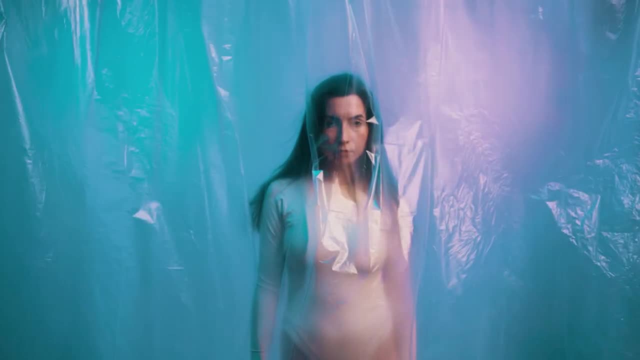 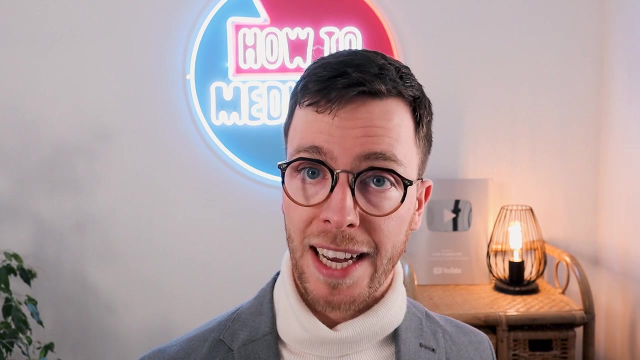 Don't use a plastic bag over your head or impede your breathing in any way. If you have a big tank with nitrous oxide, make sure that it does not come into contact with any flames or with cigarettes, as it might explode. Don't combine it with alcohol or any. 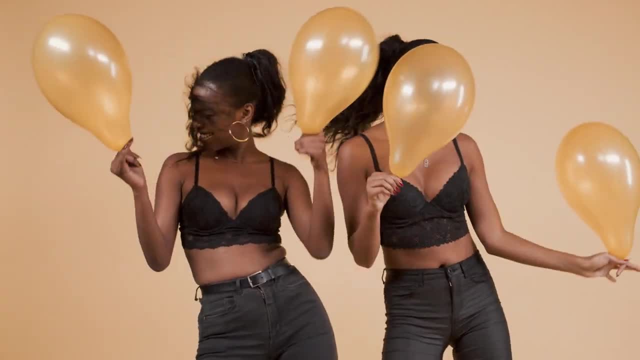 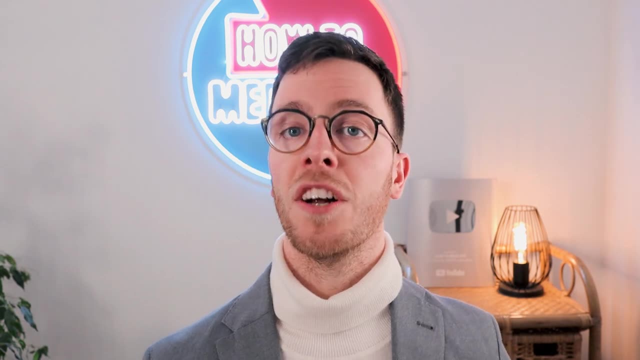 other drugs, And don't stand or dance while inhaling from a balloon, as this might increase your risk for passing out. Now I hope this video provided you with anything you needed to know on nitrous oxide. If you have any questions, let me know in the comment section and I will. 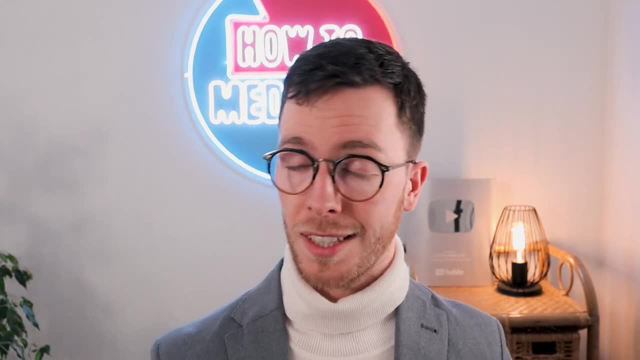 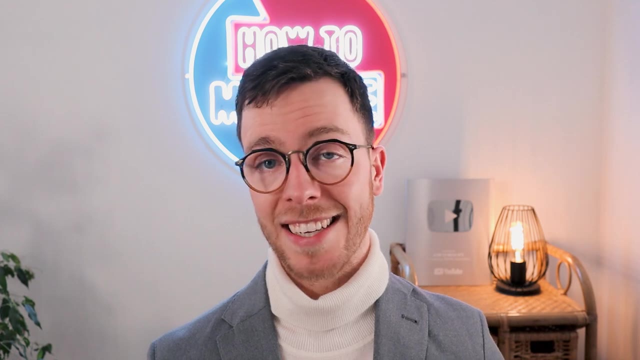 do my best to answer each and every one of them. For those of you that are still interested in learning more, I made a playlist with more videos on illicit drugs. Check it out in the description. For those of you that can't get enough, check out the Instagram, TikTok and Facebook with more.